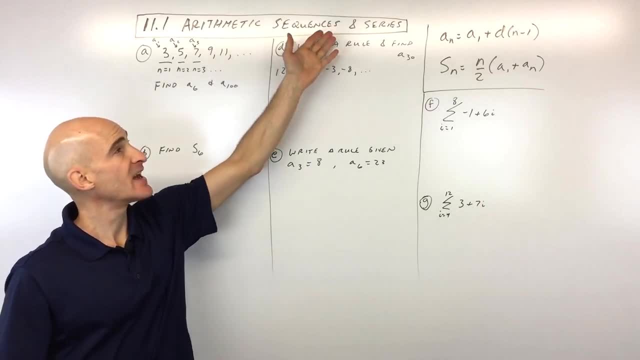 In this lesson you're going to learn about arithmetic sequences and series. So what exactly is an arithmetic sequence and an arithmetic series? Well a sequence is basically a list of 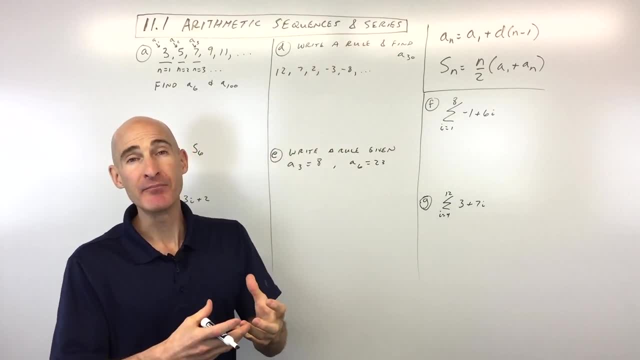 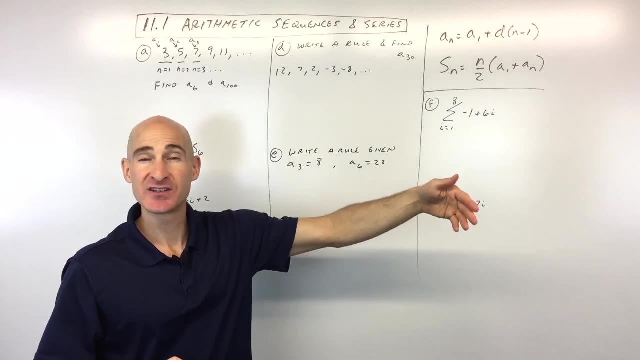 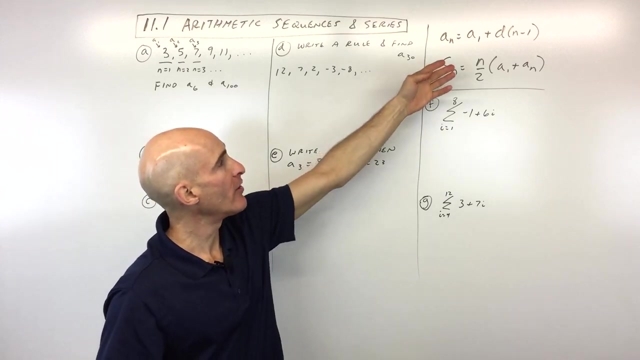 numbers and a series represents a sum of numbers. Now when we talk about arithmetic what we're talking about is that you're adding the same quantity each time to get to the next number, the next term in the sequence, and so it's a consistent pattern there. And what we call that thing that you're adding each time, we call that d, the common difference. And I'll show you 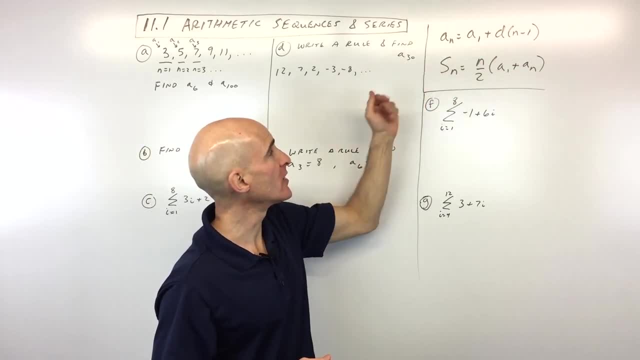 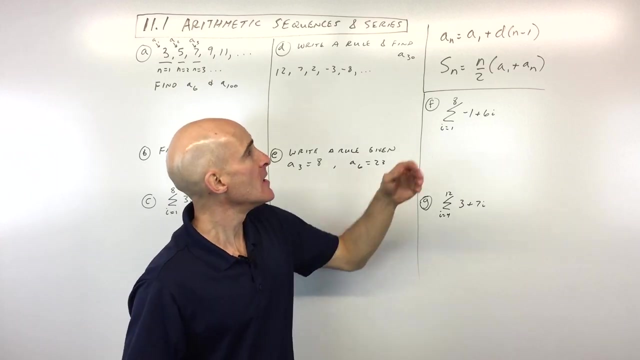 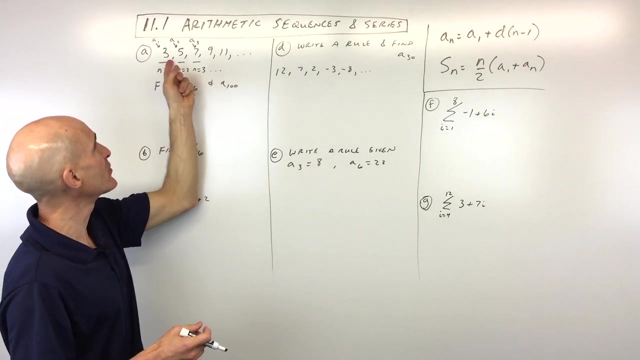 an example to illustrate how to work with these two formulas we're going to be working with here. One is the rule or formula for finding a particular term in an arithmetic sequence, that's this one here. And then the sum, if you want to find the sum of the first 10 terms, 20 terms, 100 terms, however many terms. So let me show you an example and I'll kind of go through it as we go. So for letter a here we've got this sequence, this list of numbers three, five, seven, nine, eleven, dot dot dot. So what exactly are we adding to get to the next number? 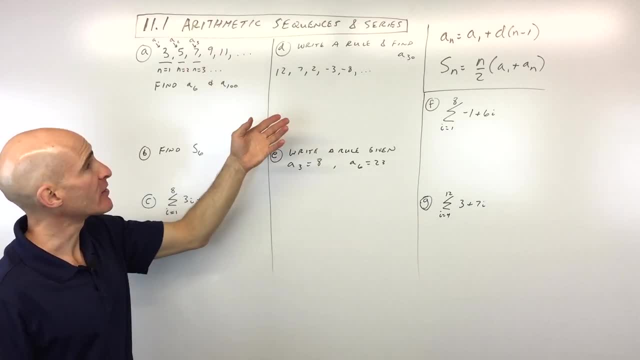 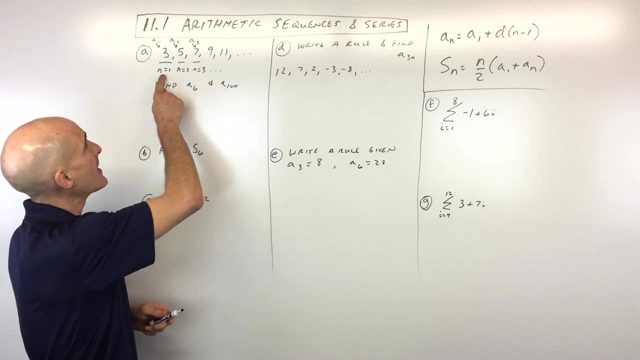 Well you can see that we're adding two and that's what we call our common difference, our d value here. Now when you talk about sequences there's a couple things you want to pay attention to. One is that you see I have written n equals one, n equals two, n equals three, 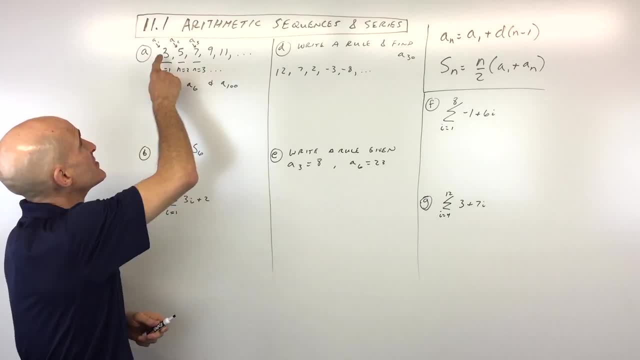 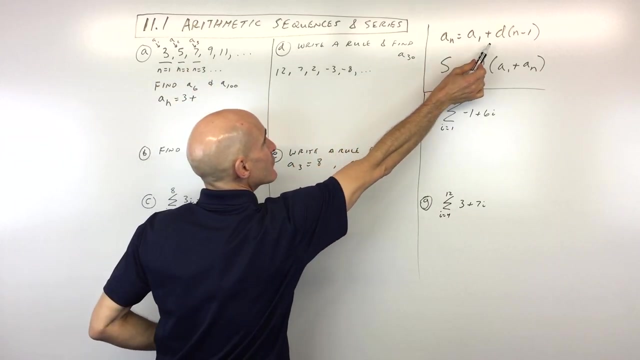 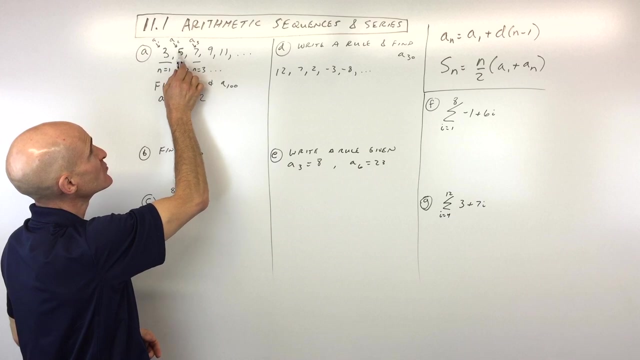 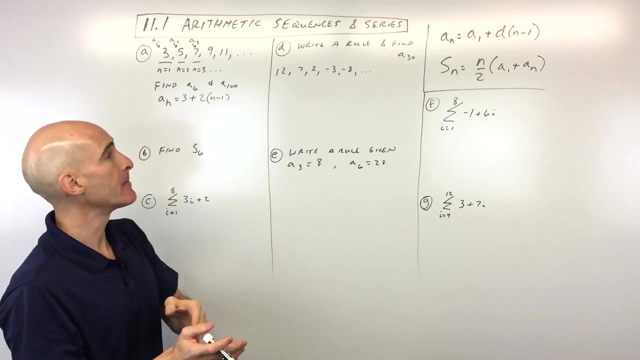 that's the term that we're talking about, the term number. But see this a sub one, a sub two, a sub three, that represents the value of the term. Now when I say sub I mean like sub subscript. So a sub one means you know one is a subscript, but it's basically referring to what's the value of that first term, what's the value of the second term, etc. So when we look at this formula, if we want to find you know a formula for this pattern here, what we would do is we'd say a sub n, meaning the value of our nth term, equals the value of the first term, which in this case you can see is three, plus the common difference. Okay you can see we keep adding that difference of two. Now the reason they call it the difference is if you take five minus three, see you know the difference between five and three, you get two, seven, eight, nine, ten, eleven, twelve, thirteen, twenty, twenty-two, twenty-three, twenty-three, twenty-three, twenty-three, twenty-three, twenty-three, seven minus five, you take the number minus the one before it, and then we've got n minus one. So this is a formula. Now if you want you can distribute the two into the parentheses here and combine like terms, but for right now I'm just going to leave it like that. 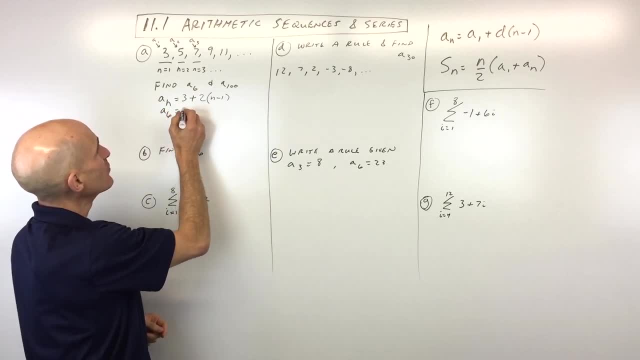 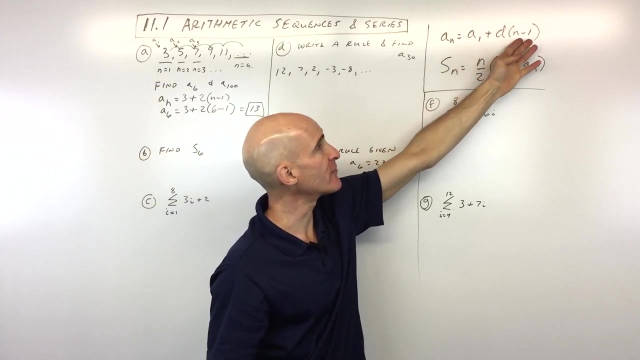 But if we want to find the sixth term, a sub six, we would take the first term which is three, plus the common difference two, and now this n tells us what term we're on, that's the sixth term we want, minus one. Six minus one is five, times two is ten, plus three is thirteen. So you can see the value of that sixth term is thirteen. Now I just want to explain a little bit how the formula works just so you can understand a little bit better. See here's one, two, three, four, five, here's our sixth term right here. But we're starting at three and we're adding two once, twice, three times, four times, five times. How come not six times? We're on the sixth term, right? Well because we already started at the first term, we only have to add that common difference n minus one times. Okay, so that's where this n minus one is coming from. We're just adding that common difference of two, five times, not six, and then we're adding that to the first term. 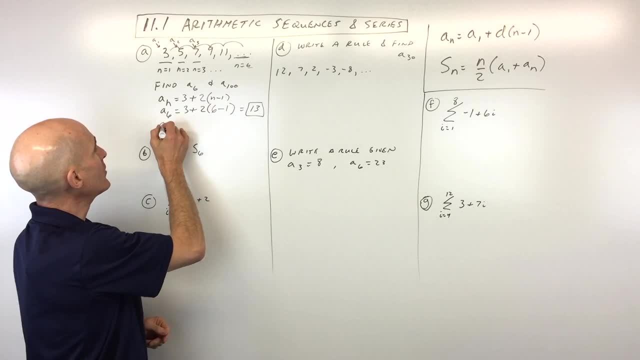 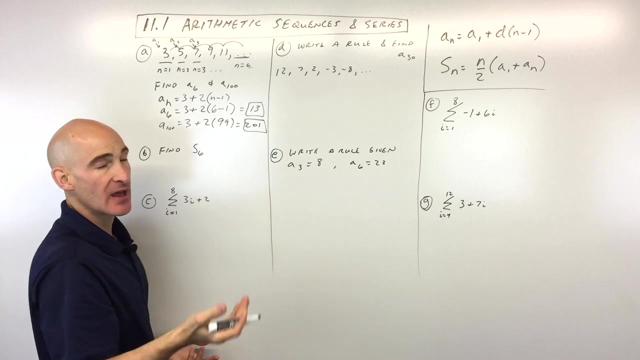 So that's where the formula comes from. Now let's do this other one, a sub 100. Well you wouldn't want to add two, you know, until you got to the hundredth term. That would take quite a bit of time. So that's where the formula really benefits you. So we start at three, that's our first term, we're adding two 99 times, not 100, 100 minus one, 99. So that's 198 plus three, which gives us 201, 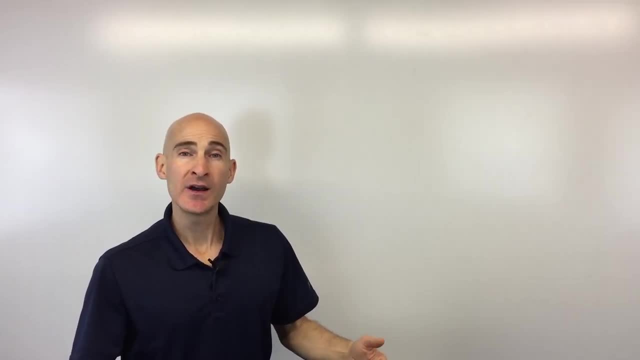 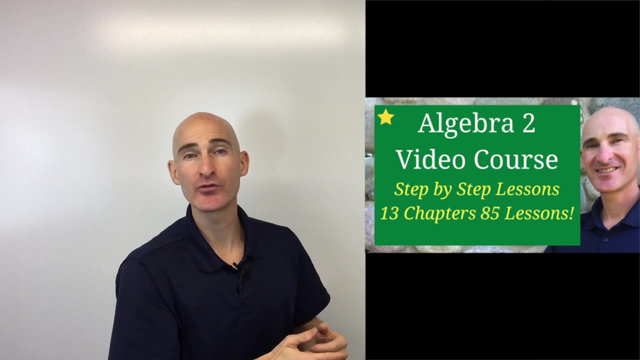 you've got it. Okay, let's go to another one. Want to learn Algebra 2? Check out my Learn Algebra 2 video course for sale where we go through 85 video lessons that take you step by step by step through Algebra 2. We go through the important formulas, concepts, as well as numerous examples to help you master Algebra 2. Click the interactive card or the link in the description below to go 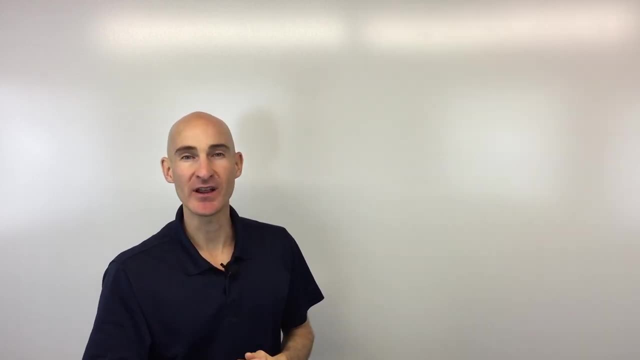 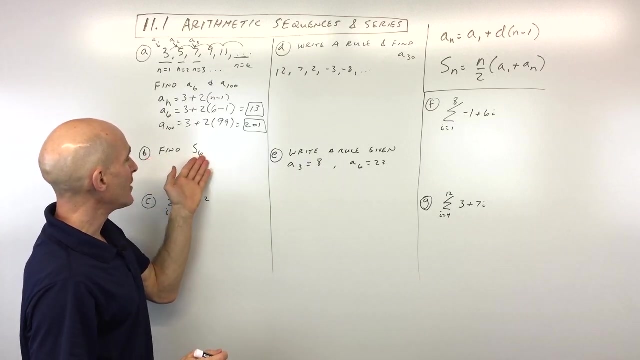 over and check out some of the free lessons. Otherwise, let's get back into this current lesson. You've got it. Okay, let's go to another example now. So for letter b, what we're going to do is we're going to find the sum of the first six terms. So see how this subscript here six tells 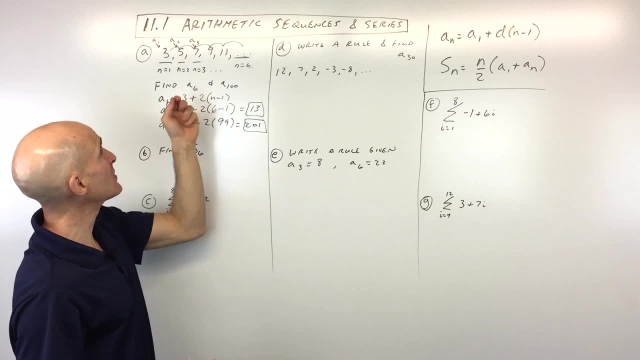 us we're finding the sum, s for sum, the first six terms. Now you might say, well, Mario, I can just go ahead and add those six numbers together. And that's fine. But what happens is say you want to find the first the sum of the first hundred terms, it would take quite a bit more time to first write them all out and then add them all up. So let's just go ahead and I want to show you a pattern 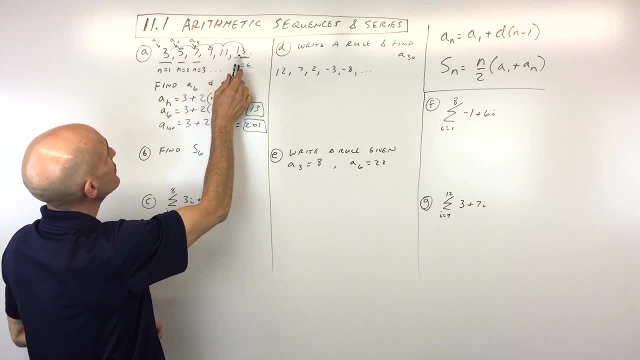 here. So notice if you add three and 13 together, you get 16. See if you add five and 11 together, you get 16. 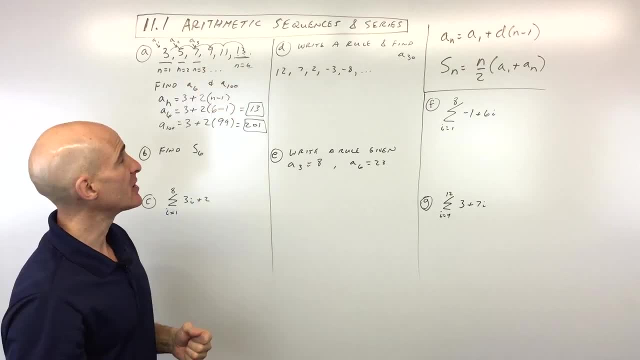 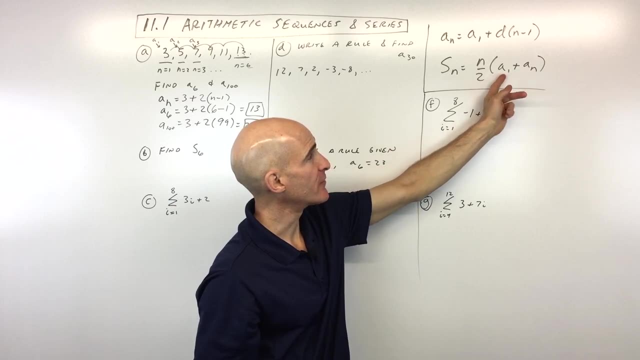 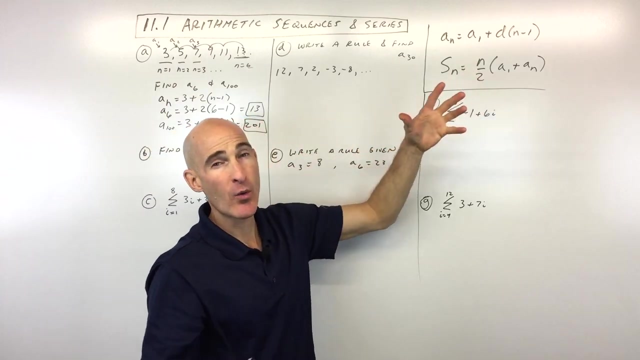 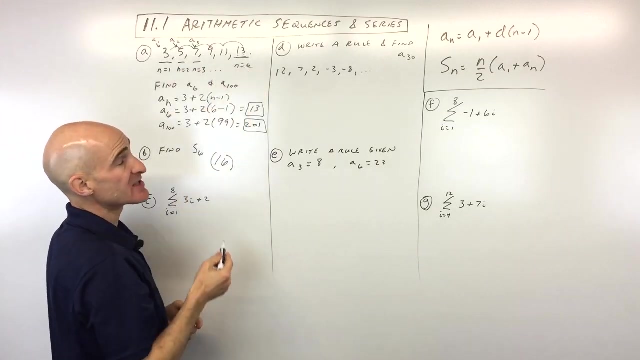 If you add seven and nine together, see how you get 16. Very interesting pattern. So what we're doing is we're taking the first term, a sub n is like your last term. So you're adding the first term for the last term. So notice we're doing three plus 13 is 16 times the number of terms divided by two. Now why the number of terms divided by two? Well, remember how we said we got 16? But how many 16s do we get? Do we get six 16s? No, we had half that many because we're pairing two numbers together each time, we're actually only getting three 16s. We're actually only getting three 16s because we're pairing two numbers together each time, we're actually only getting three 16s. 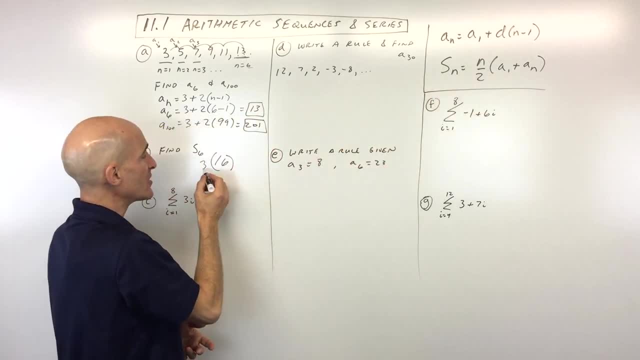 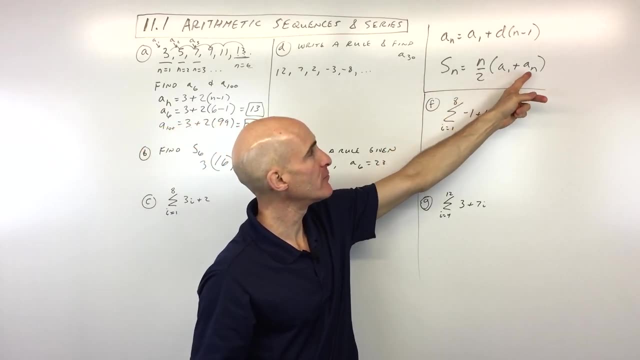 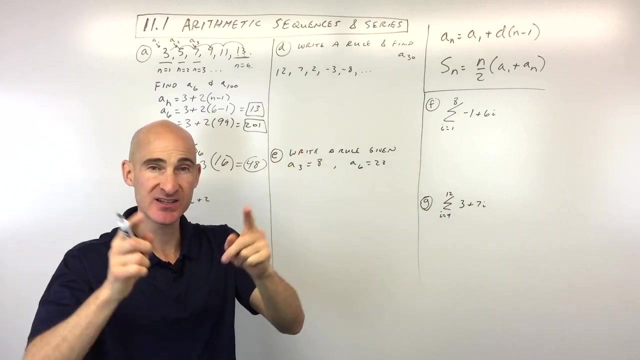 We're actually only getting three 16s. Which you can see is six divided by two, that's three. So three times 16, we get a sum of 48. So just trying to show you and give you a feel for how these formulas work. First term plus the last term times the number of terms divided by two, so half the number of terms. Because you're pairing them, you know, first and last second and second and last, you're going to have half as many of those groups. Okay, let's go down to 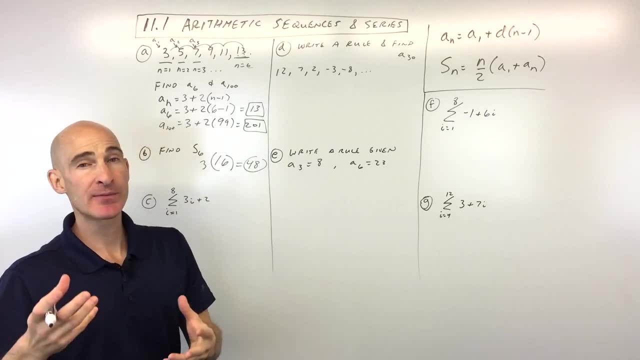 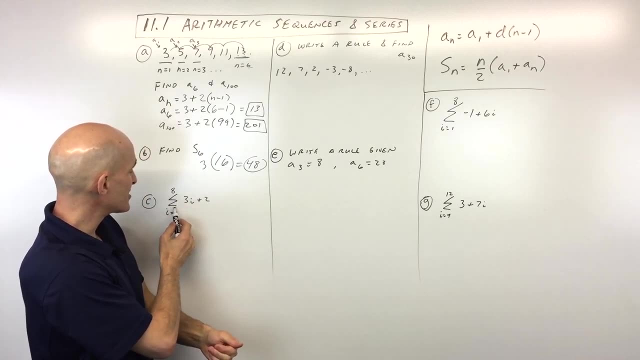 letter C. Now what we're talking about in letter C, these are all introductory examples, I'm going to have some that you can practice on your own. But to show you the notation here, see this, kind of squiggly line here, this is the Greek letter sigma. And this represents the summation or the sum. What we've done here, instead of just writing it as a list, like, like, so what we're 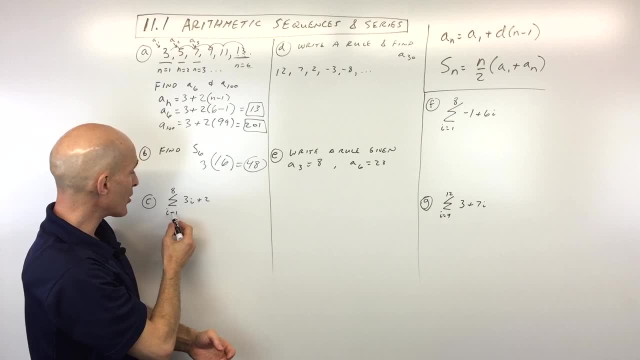 doing is we're writing it in a compact form, I is what we call our index, what you do is you start at this bottom number here, I equals one, you put it in for I here, three times one is three plus two is five, that's our first term. Now the sigma or the sum just means that you're, you're adding each term, and you work your way up sequentially from one to eight. So the next term we're going to be two, so we put two in three times two is six plus two is eight, we put the next one in three, we get nine plus two is 11. Until you get to the eighth term, dot dot dot three times eight is 24 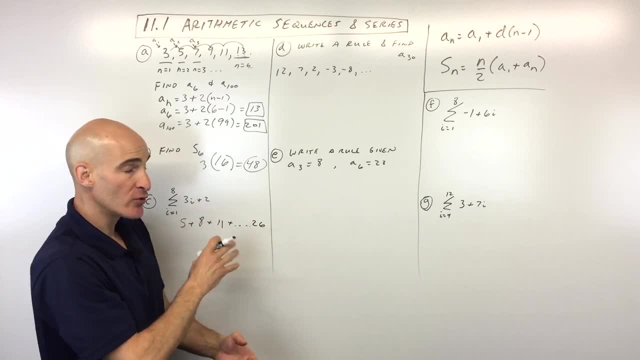 plus two is 26. Okay. And again, so all we're doing is refining the sum, this is just a compact, compact way of writing that as a summation. So they call this sigma notation. So what we want to do here is we want to use our sum formula, which is this one right here, we're finding the sum of the first eight terms, there's eight terms. So we're going to use our sum formula, which is this one right here, we're finding the sum of the first eight terms, there's eight terms, so we're 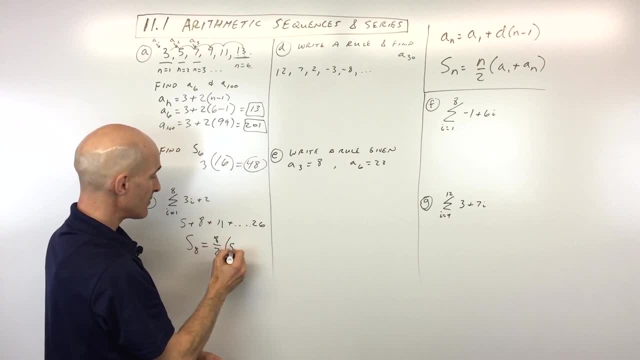 going to use our sum formula, which is this one right here, we're finding the sum of the first eight terms, there's eight terms. So eight divided by two, the first term we know is five. And the last term we know is 26. And if we simplify, you can see eight divided by two is four, five plus 26 is 31. So that gives us 124. And it saves us from having 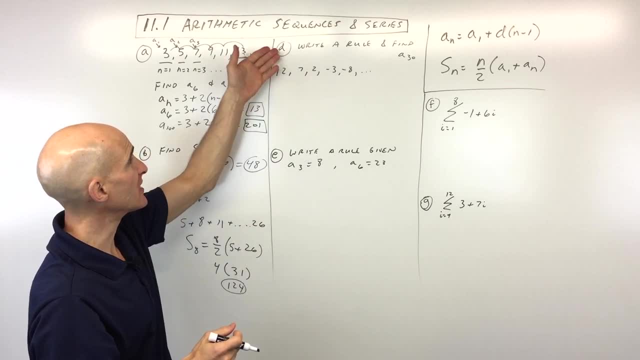 to write all those out and add them together. Okay, let's go to example D here. Now, it says 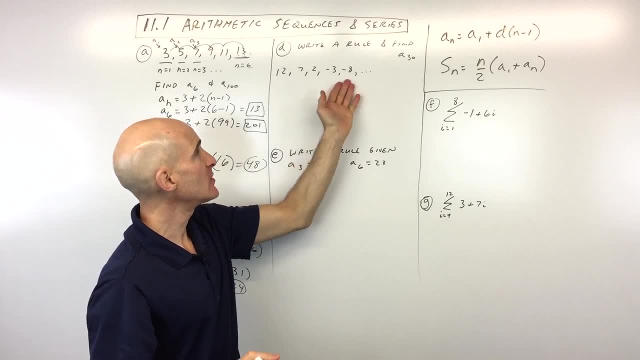 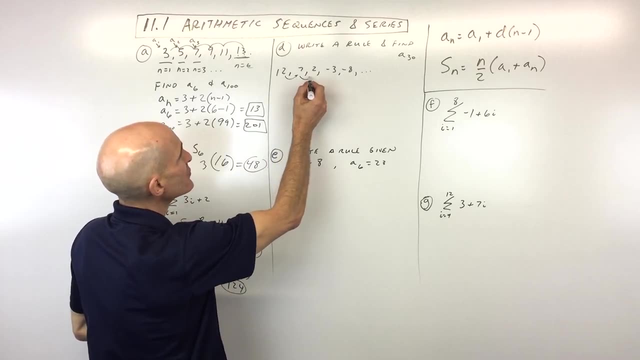 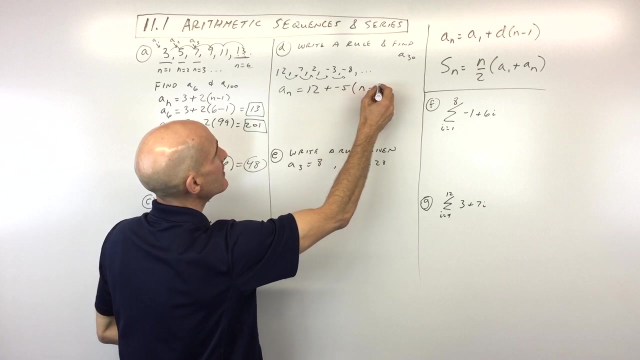 write a rule, basically, that just means like a formula for this sequence here and find the 30th term, okay, the value of the 30th term. Well, let's see the pattern here, what's what are we doing to get from the first term to the next term, etc. Well, it looks like we're subtracting five, right? So if we use our formula here, this one at the top, we've got our first term is 12. Our common difference is a negative five, you could write minus five or plus a negative five times n minus one. Now here, what I'm going to do is I'm going to distribute the 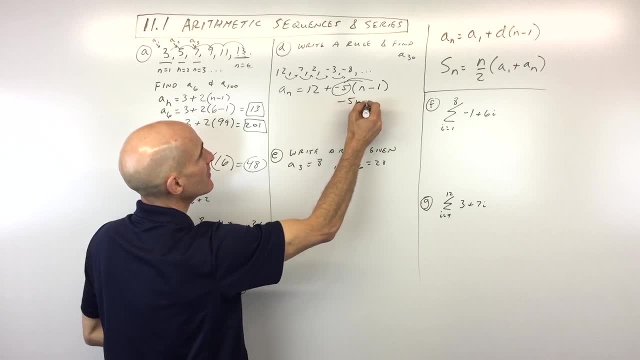 negative five, I'm going to simplify this down a little bit for us. So negative five n plus five, plus 12. So this comes out to negative five n plus 17. That's a formula for any term. Now, if we want to find the 30th term, a sub 30, we're going to put 30 in for n. 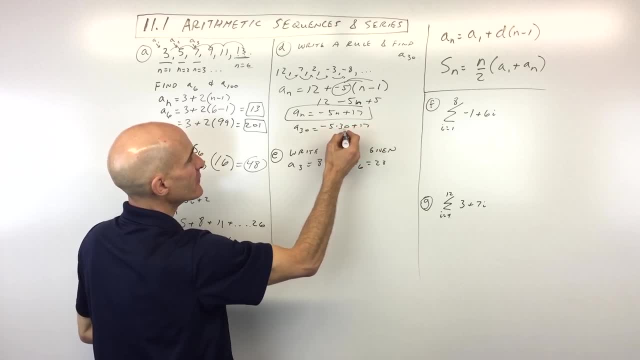 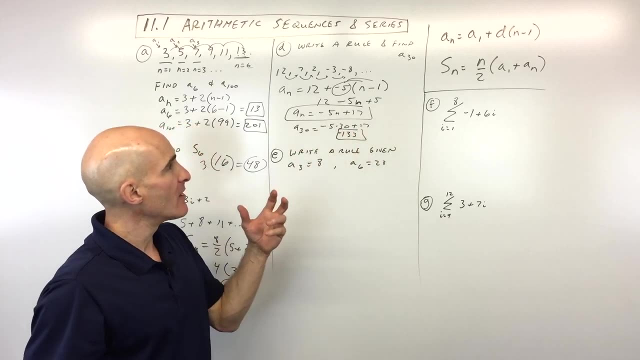 So negative five times 30. That's a negative 150 plus 17 is what 133. And it'll be negative. So don't get confused when you see these subscripts. See this, this doesn't mean s times n, 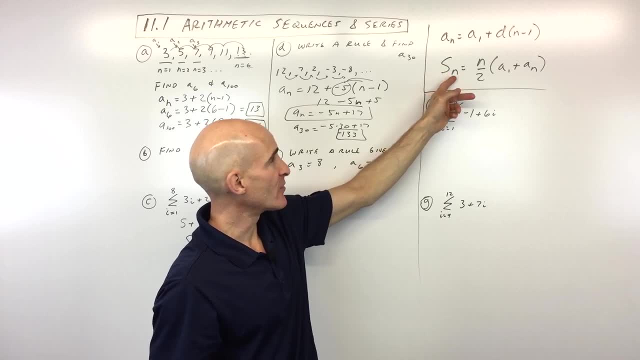 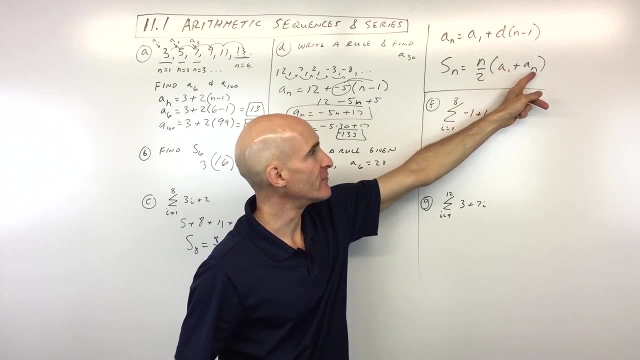 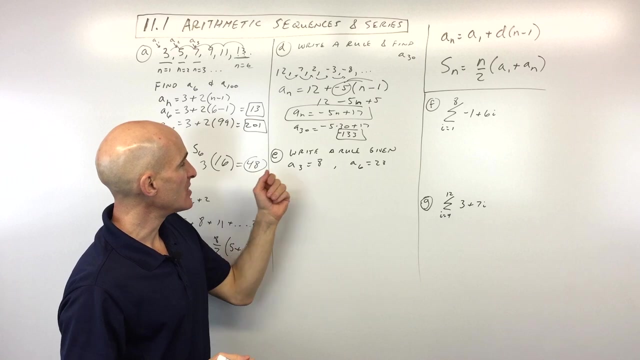 it's really telling you Oh, that's the nth. That's n number of terms that we're finding the sum for, you know, same thing here. It's not again, it's not like eight times n or eight times one, this is the value of the first term, the value of the nth term, or in this case, it's the nth term represents the last term that we're trying to find the sum of. Okay, let's look at example E 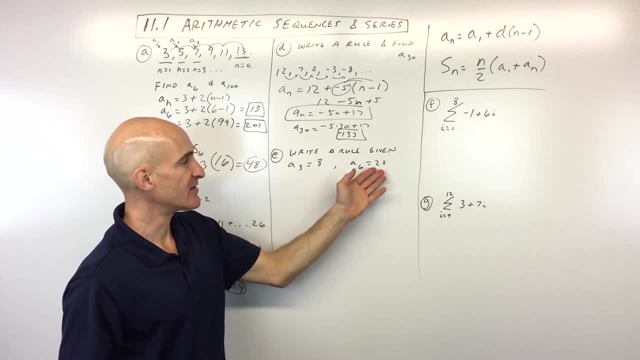 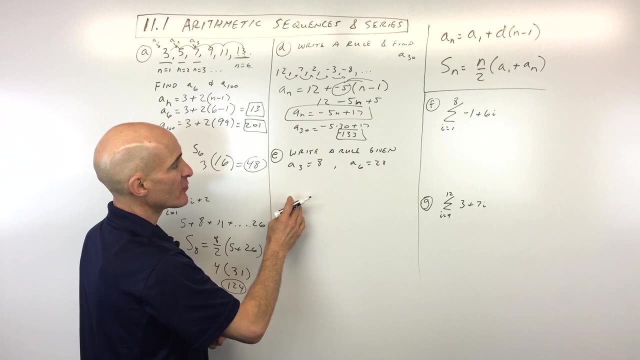 here. It says write a rule given that the third term is eight and the sixth term is 23. Okay, so this is very interesting. We've got two pieces of information about the sequence, we've got one, two, the third term is 845. The sixth term is 23. Now there's a lot of different ways to do these 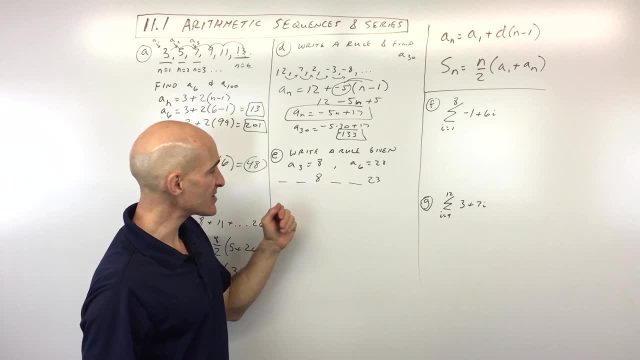 problems. Assuming this is an arithmetic, a sequence here, we could just say, well, eight plus D as our common difference plus D again, plus D again, we could say eight plus three D equals 23 and solve that for the common difference. 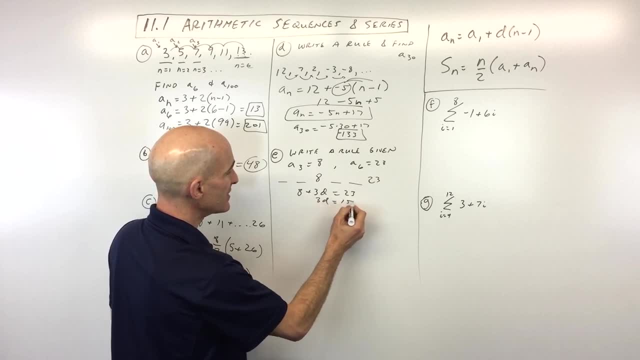 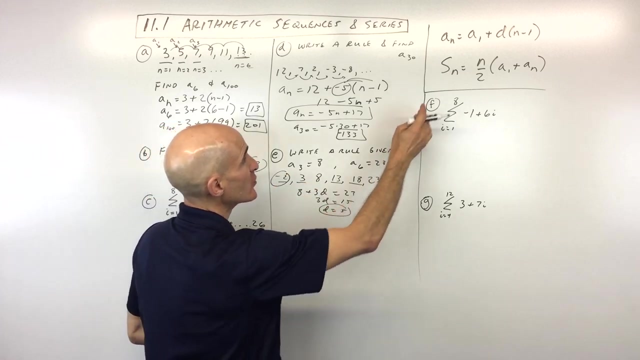 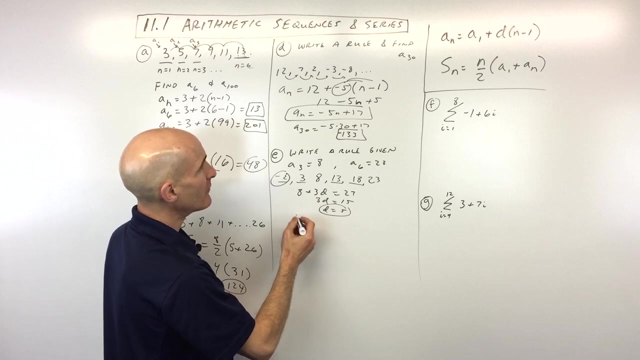 So here, I'll do that as three D is equal to 15. So you can see D is equal to five. So that means we're adding five. So this would be 1318 23. And if we worked our way backwards, this would be then be three, and this would be negative two, right? So now we have the first term, we have the common difference, we could write our formula. Sometimes they're not so easy like that. So what I want to show you is another method. And that's what I'm gonna do is I'm going to write a system of equations. So what we're going to do is the first term we know is well, let's pretend we don't know the first term, okay, say it's a sub one, the common difference, we also don't know. But let's say we know the third term. So three, minus one is two, right? And the value of that third term is eight. So that's our first equation. The second one, we know the 23 is the value of the sixth term. So 23, I'm putting in the value of the sixth term, the first term, let's say we don't know the difference, let's say we don't know. But we know that six minus one is five. So now we've got two equations with two variables, a sub one and D, what I'm going to do here is I'm just going to subtract, okay, using the elimination method. So the A ones are going to cancel, two D minus five D is negative three D eight minus 23 is negative 15. If I divide by negative three, you can see D equals five, same thing we got here. 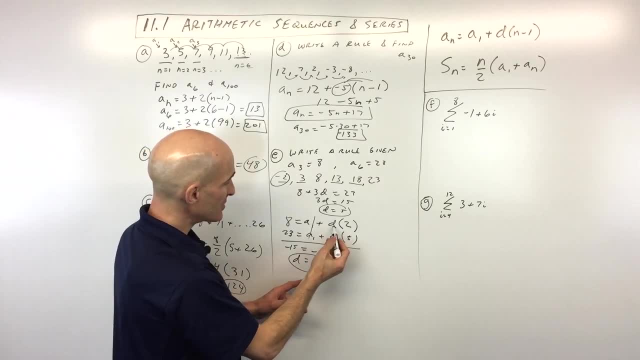 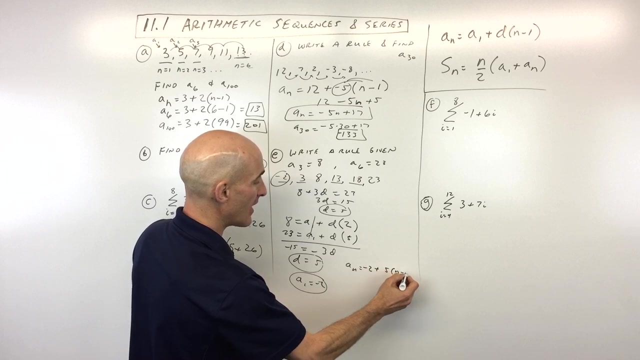 Okay, just doing it a different way. If we put five back in, I'll put it into the top equation, that's going to be 10. If I subtract 10, you can see that a sub one is equal to negative two. So now if we put it all back together into a formula, we've got a sub n equals our first term, which is negative two, and we keep adding five and minus one times, we can simplify this 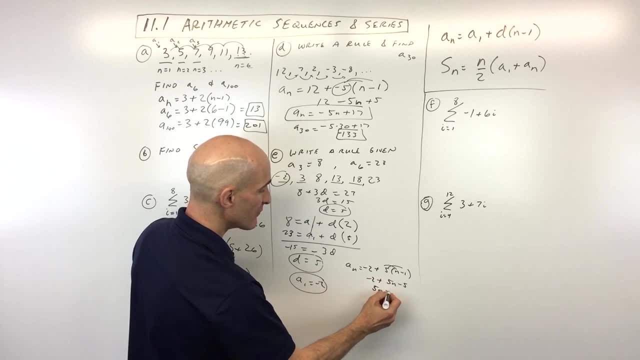 a little bit five and minus five, combined like terms, we get five and minus seven. That's our formula. If you want to test it out, let's see the sixth term would be 30 minus seven. 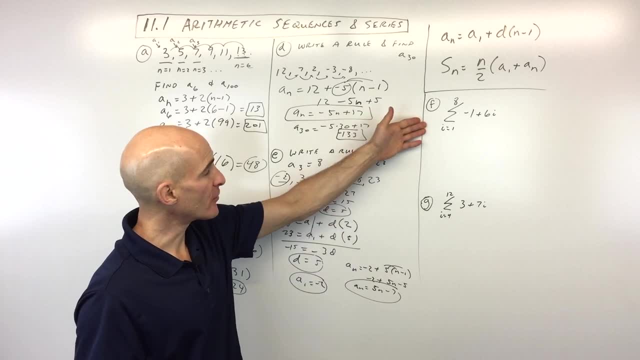 That's 23, you know, you can verify. Okay, let's go to letter F and letter G. Now, we're doing some more summations here, you can see, notice for this one, we've got 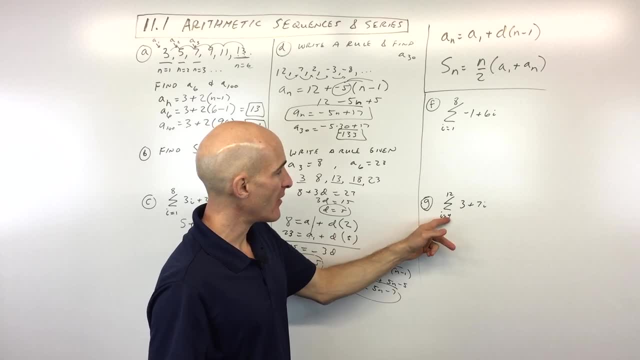 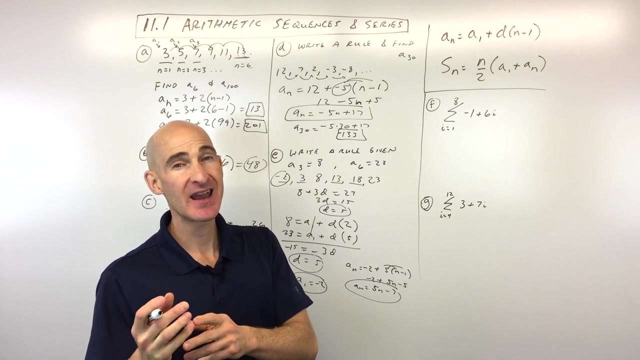 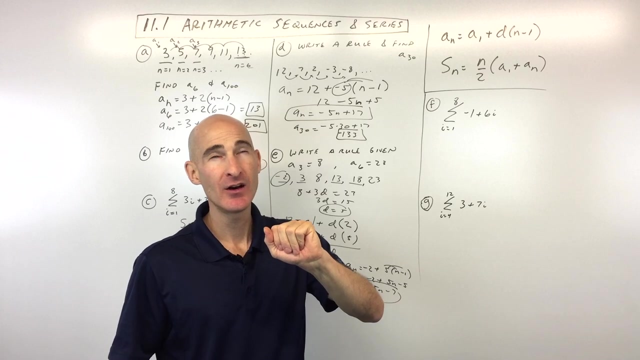 eight terms one through eight. Whereas for this one, you see we have how many terms from four to 12. So you start at that bottom index, you work your way up sequentially to the top number here, how many numbers do you think there are between four and 12? Well, if you said eight, you're close, it's actually going to be nine. And the reason is, if you count the first number in the last number, like, say, if I say how many numbers are there from one to five? Well, five minus one is four, right? But you can see there's five, five numbers there. So when you subtract, you want to add one more if you're counting the first and last term 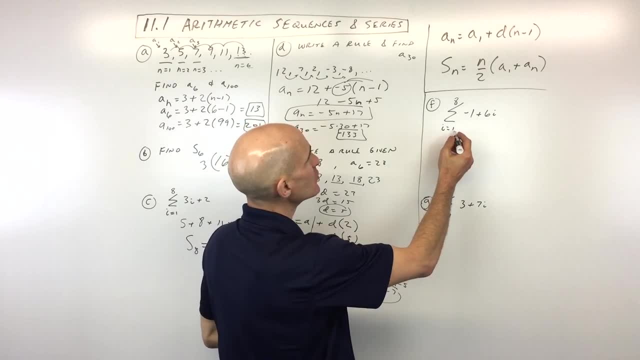 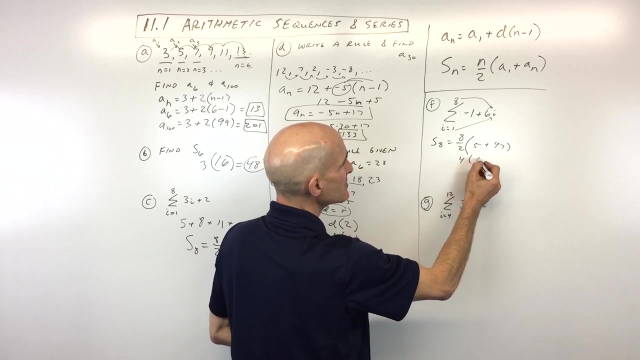 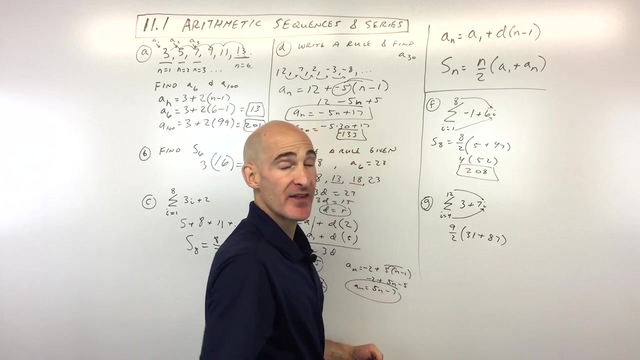 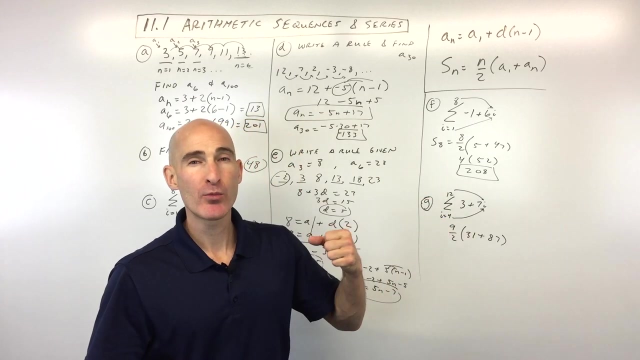 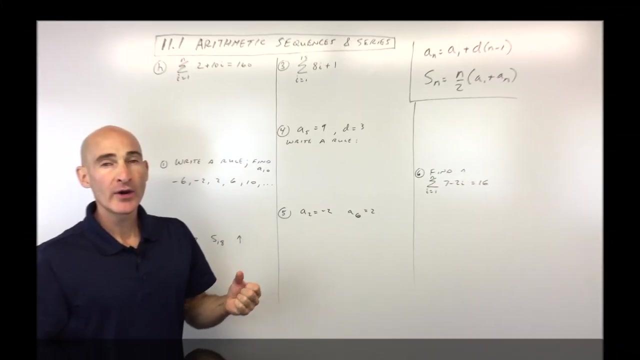 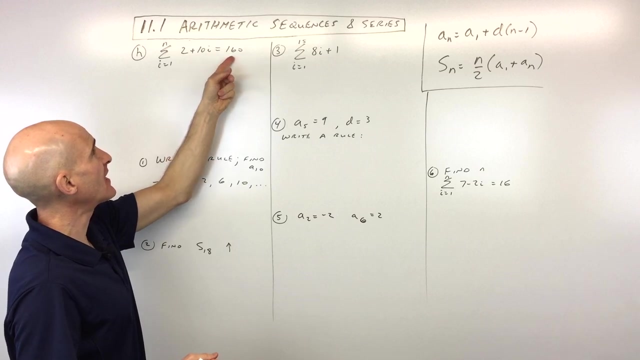 like that. So just a just a note there. So let's see if we can do this one. So we've got eight terms. So we're going to find the sum of the first eight terms, eight divided by two. Now the first term, how do we find the first term, we put one in, okay, so negative one plus six is five, how do we find the nth term, or in this case, the eighth term, that's the last term, we put in eight, it's 48 minus one, which is 47. So we have four times 52, which is 208. Okay, for letter G, same thing you can see here, we said there's nine terms. So it's nine divided by two, the first term we're going to put in is four. So that's 28 plus three, which is 31. And we put the 12th term in for to get the last term, that's 84 plus three, which is 87. And you can see this, if you simplify that, that's going to give you the last term. So we're going to put the last term in, and we're going to value of the sum of the first, well, not the first, but the terms from four to 12. So let me erase the whiteboard, I've got one more introductory example. And I've got some problems you can practice on your own. So you can get some more experience. Okay, letter H, we've got a summation here, i equals one to n of two plus 10 i and that sum equals 160. So here, what we have to do is we have to work backwards and find out the number of terms that are in this series. So what we're going to do here is we're going to look at our formula, we know that the sum is 160. We know the number 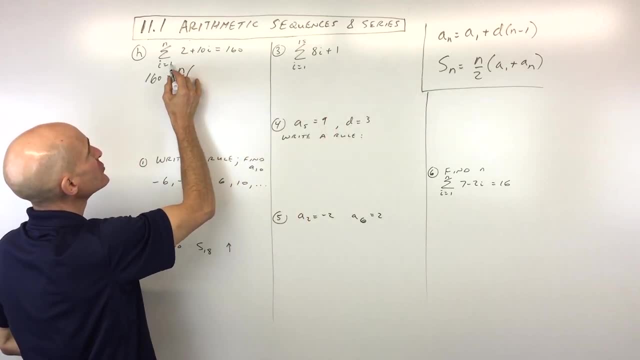 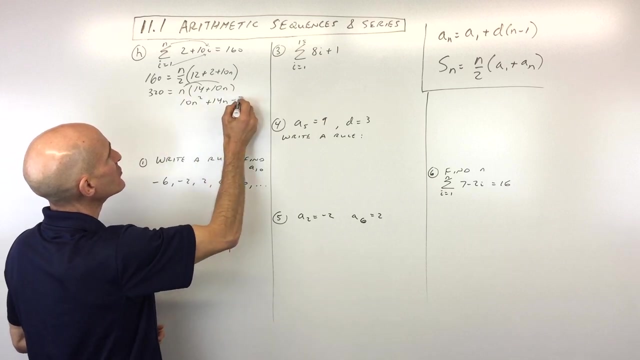 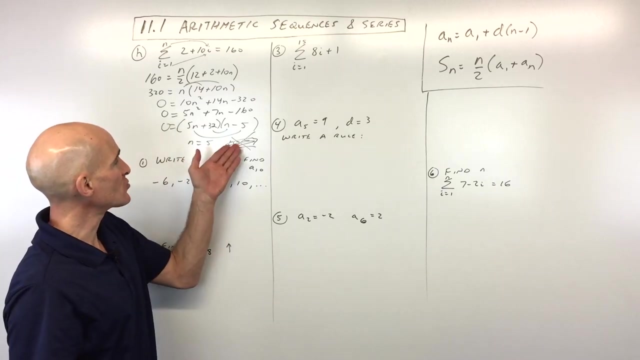 of terms right now is n, that's what we're actually solving for. The first term, if we put one in, you can see that's going to be 10 plus two, which is 12. And the last term a sub n over here, we're going to put n in, we get two plus 10 n. Okay, so all we have to do now is solve this equation for n and we've got it. So let's simplify a little bit here. I'm going to multiply both sides by two to get rid of this two. So that's going to be 320 equals n times 14 plus 10 n. If I distribute the n, I get 10 n squared plus 14 n. I'm going to subtract the 320 to this side so we can set everything equal to zero. Now you could do the quadratic formula or you could factor. Let's see, I'm going to factor this. Let me see how would this factor well. First, I'm going to divide everything by two to make it a little bit easier. So five n squared plus seven n minus 160 equals zero. And if we factor this, it should factor to, let's see, 32 and negative five. So 32 n and negative 25 n adds up to seven n. So if we set these groups equal to zero, you can see that n is going to equal five or n is going to equal negative seven. Now we can't have a negative number of terms. That doesn't make any sense. Actually, that's not negative seven. That's actually like negative 32 fifths. But we can't have a negative number of terms. So we can see that's extraneous. It's just going to be n equals five. There's five 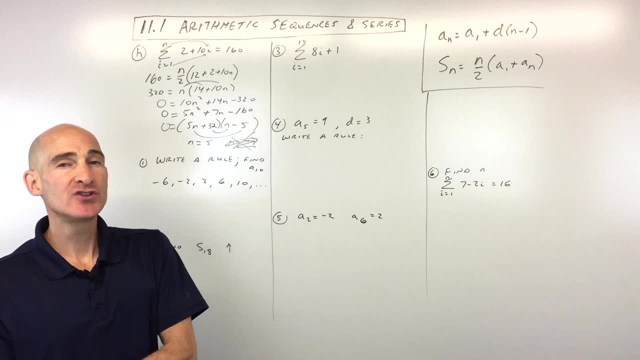 terms in the sequence and you got it. Okay, so here's your opportunity to practice. So pause the video, see if you can do the problems on your own, get some practice, and then we'll go through them. 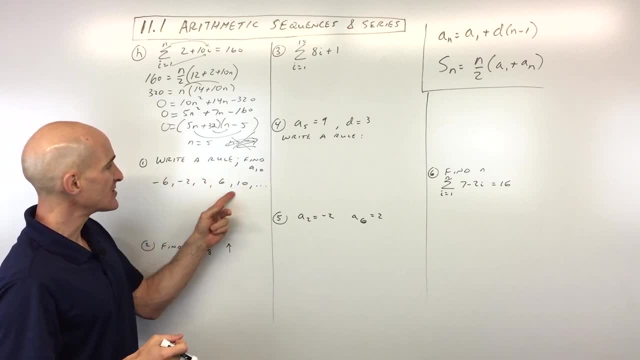 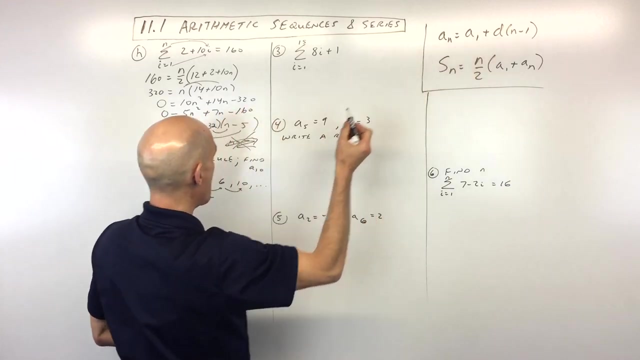 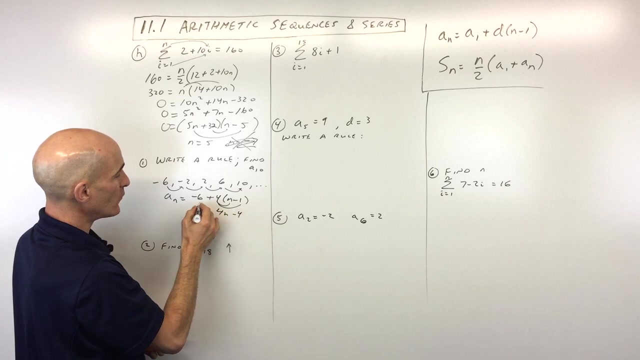 So the first one, it says, write a rule for this arithmetic sequence we have here and then find the the value of the tenth term. So how would you do that one? What do you think? Well, if I was doing this problem, the first thing I would do is I'd look to see, you know, what's the pattern? You know, what are we adding to get to the next term? It looks like we're adding four. So our formula is going to look like this. a sub n equals a sub one, which is negative six. I'm just using this formula right here. The common difference is what we're adding to get to the next term. That's four times n minus one. I'm going to distribute the four. That gives us four n minus four. 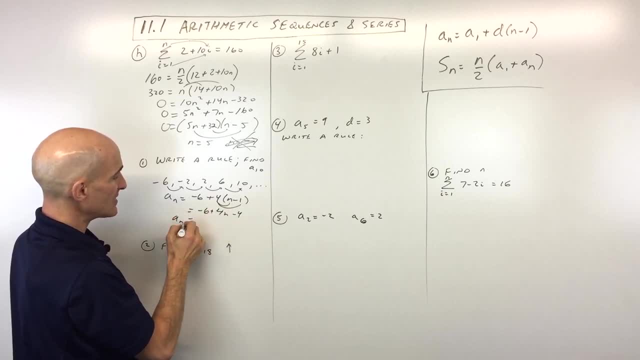 And if we combine like terms here, you can see that's going to come out to sub n equals four n minus ten. Now, sometimes I like to check my work just to see if I'm on 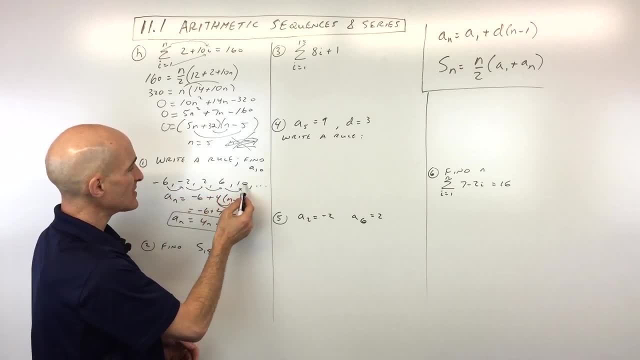 the right track. So if I put in, let's see, one, two, three, four, let's say the fifth term, 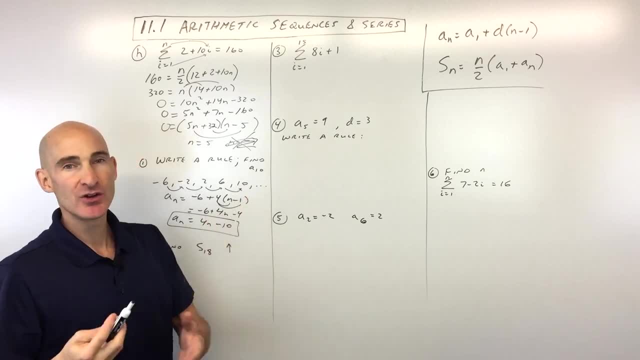 four times five is twenty minus ten equals ten. You know, it checks out. Okay, how would you do 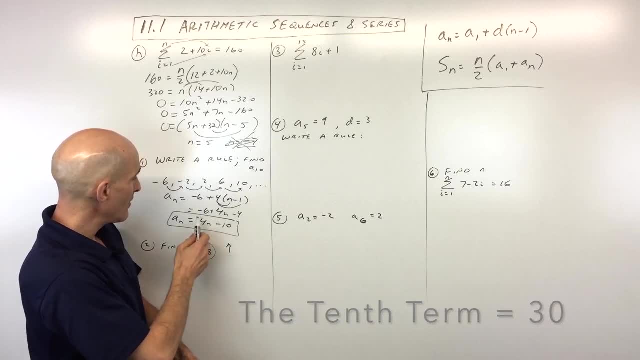 number two? Now for number two, what we want to do is we want to find the sum of the first eighteen terms. So we're treating this as a series now. A series means a sum as opposed to a sequence, 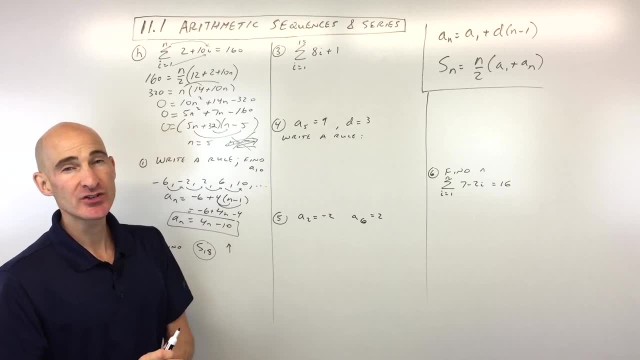 which is just the list. So what would the sum be of the first eighteen terms? What do you think for that one? 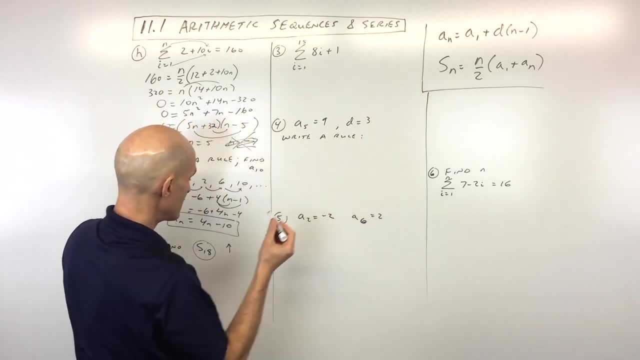 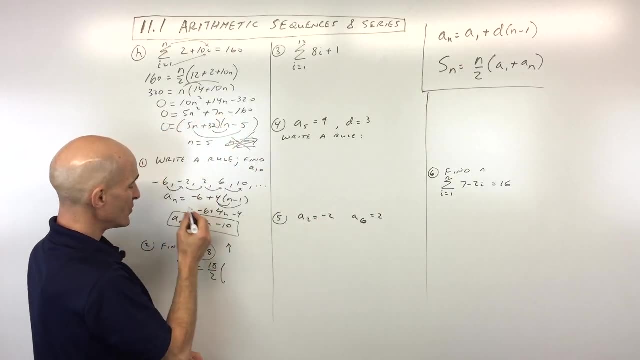 Okay, if I was going to do this one, I would use this formula right here. The sum of the first eighteen terms is going to be eighteen divided by two, because n is eighteen. A sub one is our first term, which we know is negative six. And then our eighteenth term, we have to put in eighteen here. That would be four times eighteen, which is how much? Seventy-two minus ten, which is sixty-two. So eighteen divided by two is nine. This comes out to, what is that, fifty-six. 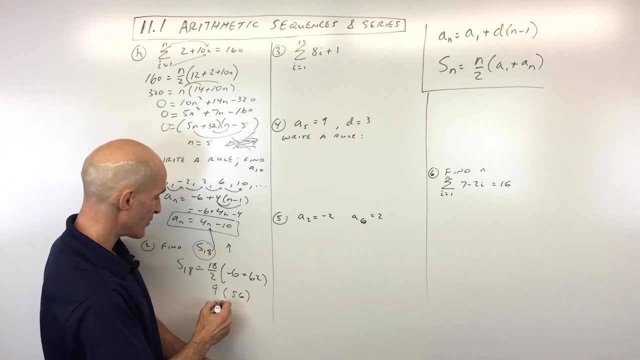 Is that right? Okay, and then nine times fifty is four hundred. Fifty, and nine times six is fifty-four. So it looks like we're coming out to a sum of five hundred 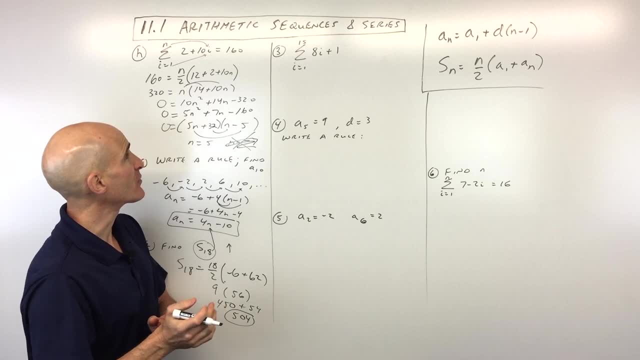 and four. Okay, so that's the key for that one. So for number three now, we've got our summation 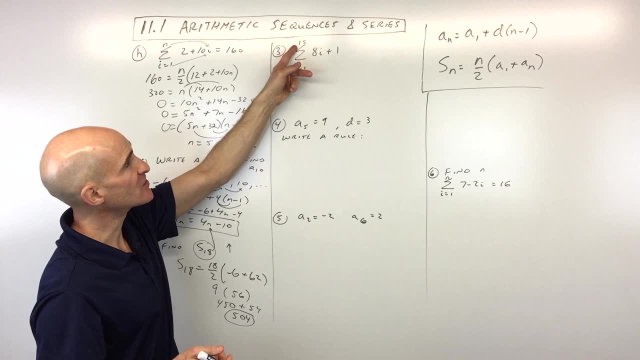 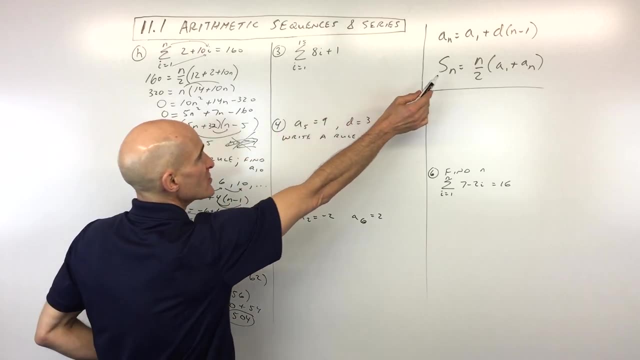 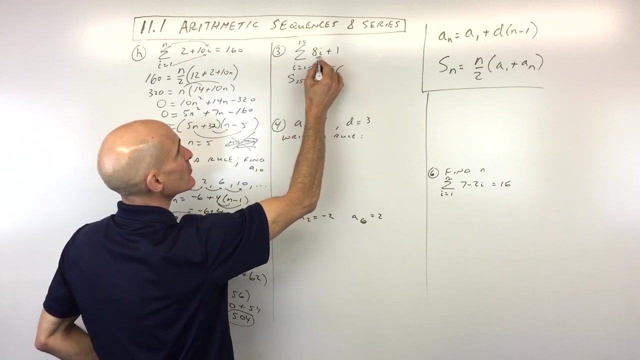 notation. We're trying to find the sum of the first fifteen terms of this series. What do you think for that one? How would you do that one? Well, if I was going to do it, again, I would be using this formula here. We've got the sum of the first fifteen terms. So we have fifteen divided by two. The first term would be eighteen divided by two. The sum of the first fifteen terms would be fifteen divided by two. The first term would be eighteen divided by two. The first term would be 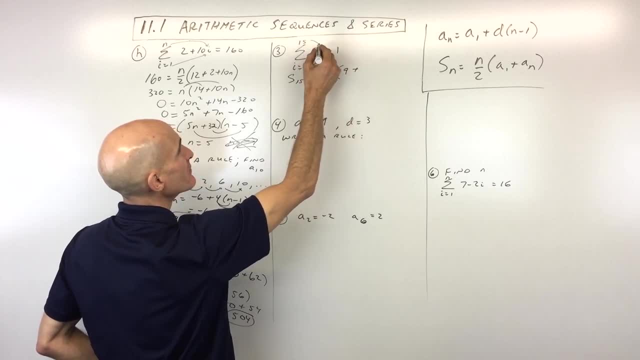 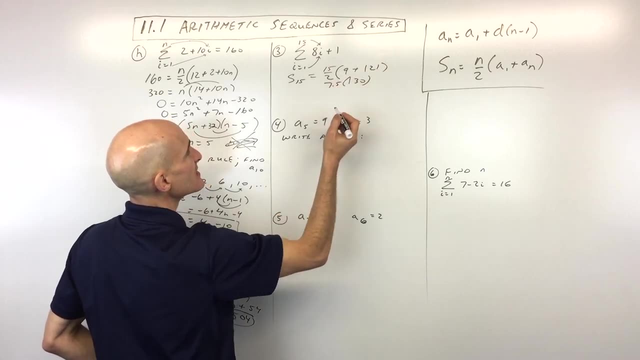 eight times one is eight, plus one is nine. The fifteenth term is going to be eight times fifteen, which is a hundred and twenty, plus one is a hundred and twenty-one. So that comes out to a hundred and thirty times seven point five. Or let's do it this way. Instead of seven point five, 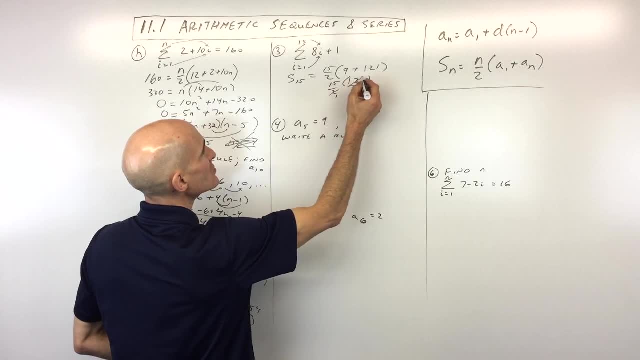 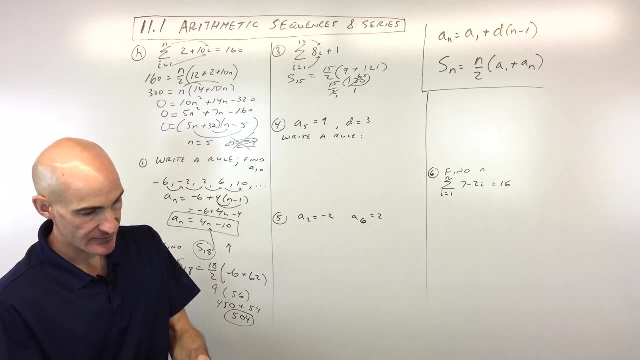 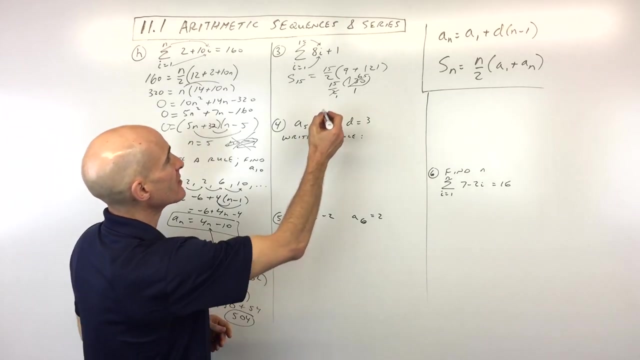 we'll do fifteen over two. Two goes in here once, two goes in here sixty-five times. So it's fifteen times sixty-five. Let's calculate that. Fifteen times sixty-five. It looks like we're getting nine hundred and seventy-five. So check your work on that one. Check my work, I should say, 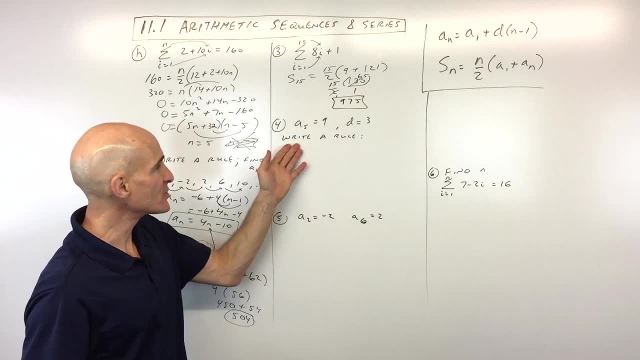 on that one. Okay, let's go to the next one, number four. So this one, the fifth term is nine. 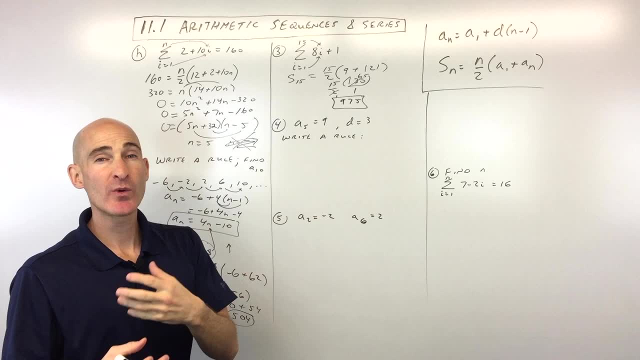 The common difference is three. This is an arithmetic sequence. We want to write a rule for any term in that sequence. So what we're going to do is we're going to use this formula here. 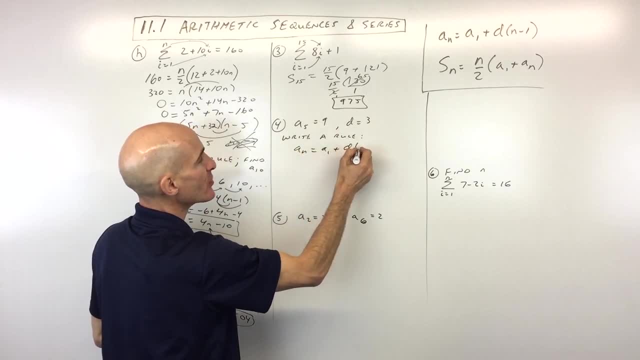 We've got, sometimes what I like to do, and this is just a good hint just in general when you're doing some of these math problems, is, you know, write down the formula first. 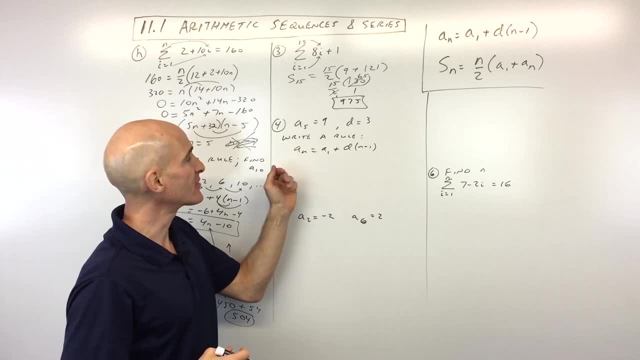 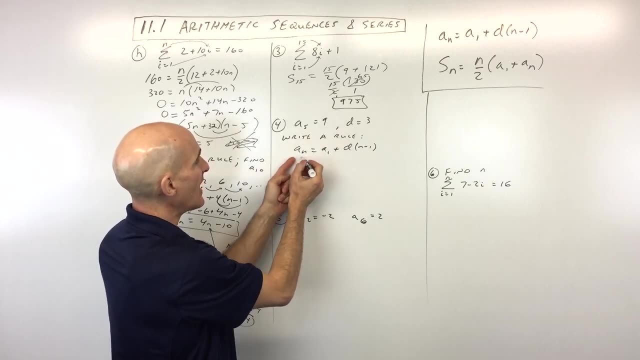 Number one, to help you memorize it. Number two, to kind of organize your thoughts. Number three, so you can kind of substitute in what you know and then you can solve for what you don't know. So in this case, we know that the fifth term is nine. So I'm going to put that here. The first term I don't know, the difference they gave us was three. And let's see, we're working with the fifth term, so this is five minus one. So it makes it a little bit easier than trying to do it all in your head. Four times three is twelve. 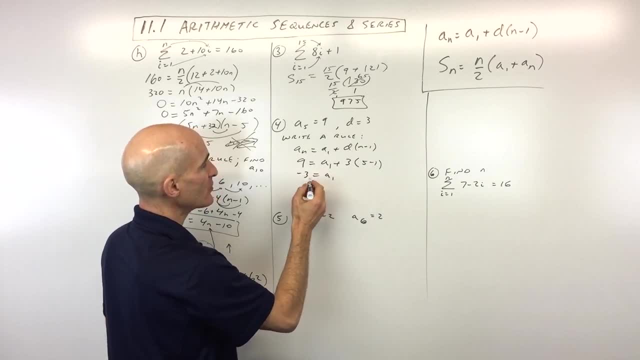 If I subtract twelve, I get negative three. So the first term is negative three. If we put that back in, now we can write our formula so we have negative 3 is the first term the common difference is 3 and if we simplify we get 3n minus 3 minus 3 okay so if we put that all together we get a sub n a sub n is equal to 3n minus 6 now i always like to check my work a little bit 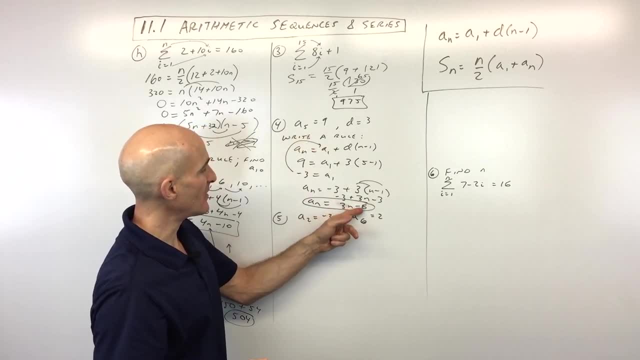 just to see if i'm on the right track so let's just put 5 in here that's 15 minus 6 is 9 okay so we can see we didn't make any little arithmetic errors or anything like that 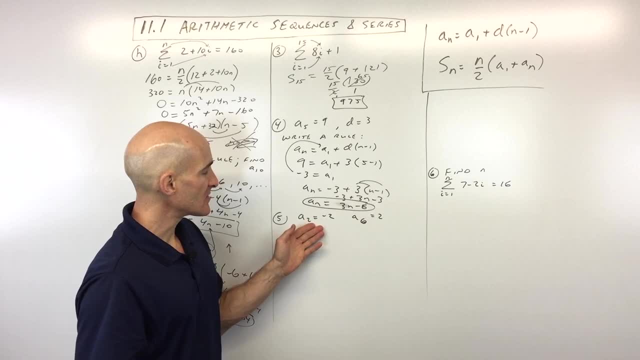 okay try number five now so here they're giving us the second term is negative 2 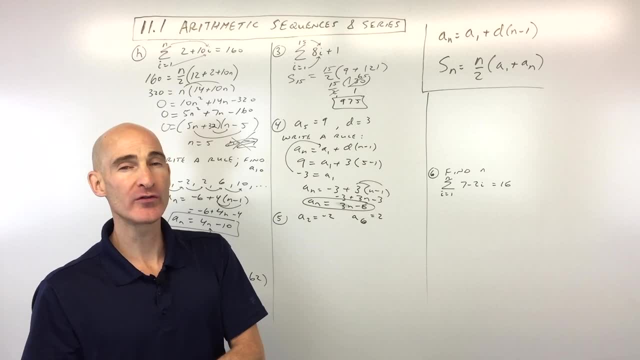 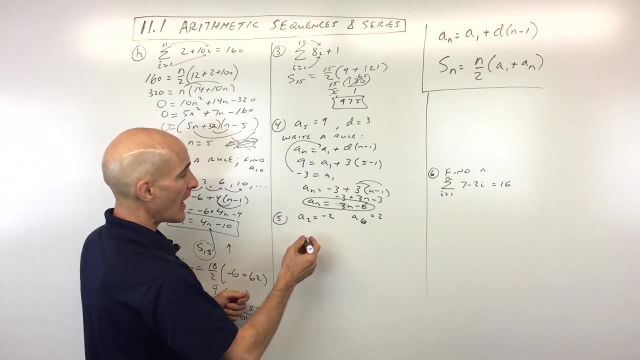 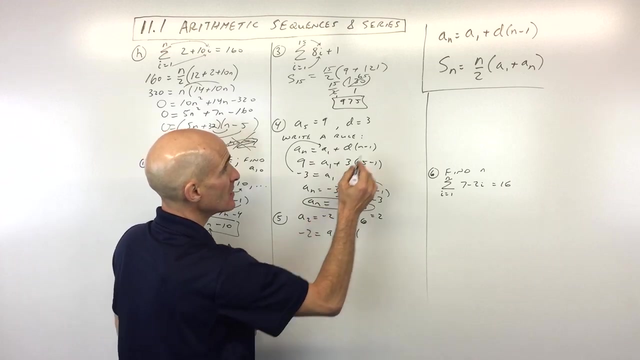 the sixth term is positive 2 how can we write a rule for this arithmetic sequence given those two terms go ahead and pause the video see if you can do that one if i was going to do it i would write a system of equations i would say negative 2 equals a sub 1 plus d times 2 minus 1 which is 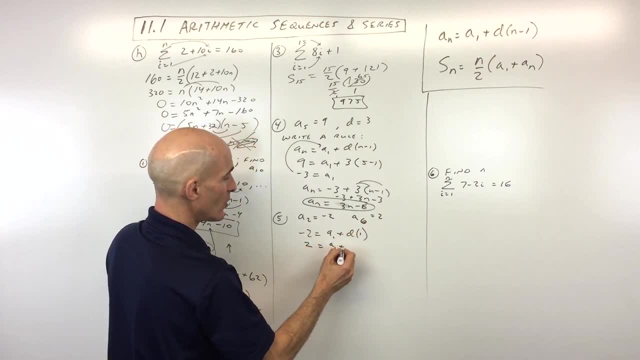 1 and the sixth term is 2 so a sub 1 plus d times 6 minus 1 which is negative 2 and we say 2 minus 1 is equal to a sub 1 plus d times 2 minus 1 which is 1 and is 5. If we subtract, negative 1 minus 2 is negative 4. These a sub 1's cancel. 1d minus 5d is negative 4d. And if we divide by negative 4, you can see that common difference is 1. 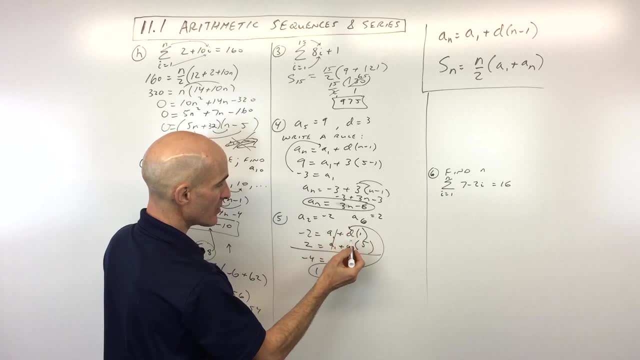 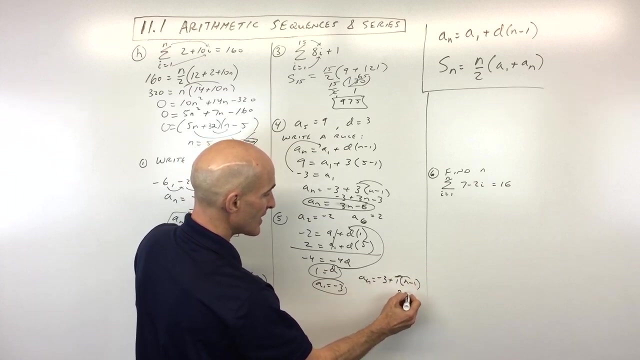 If we put 1 back in for d, let's say right here, 1 times 1 is 1. If I subtract the 1, you can see a sub 1 is equal to negative 3. So now if we put it all back together, the first term is negative 3. The common difference is 1. And we can distribute the 1. That's n minus 1. So that gives us n minus 4 equals a sub n. So if we want to check it out, let's test. So the second term 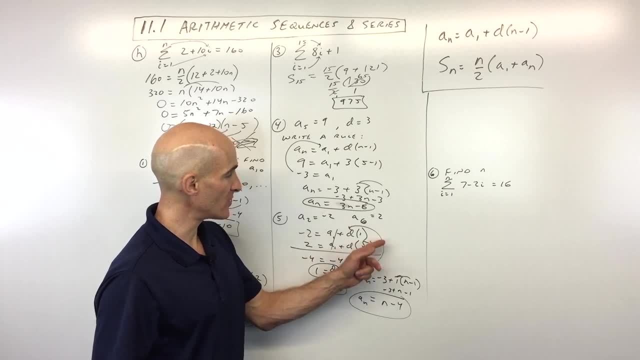 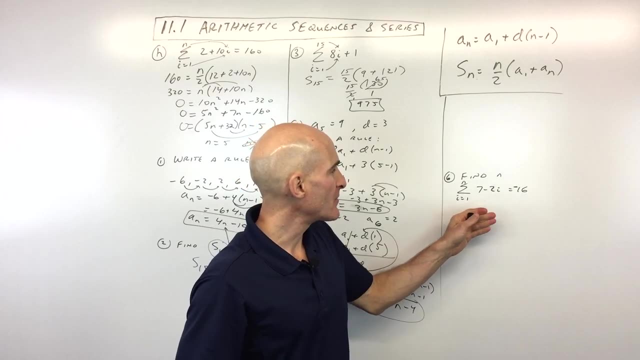 would be 2 minus 4 is negative 2. The sixth term, 6 minus 4 is 2. So you can see we've got a good formula for the sequence here. Okay, this last problem on number 6 here, I made a mistake when 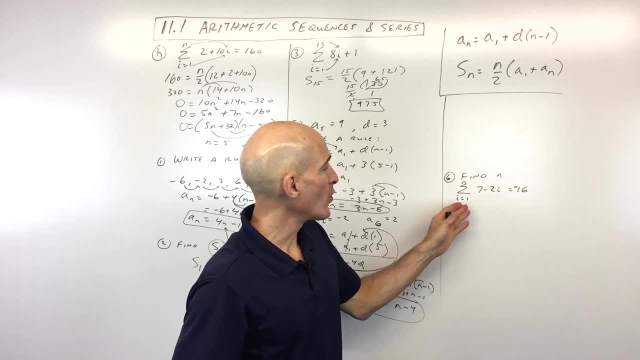 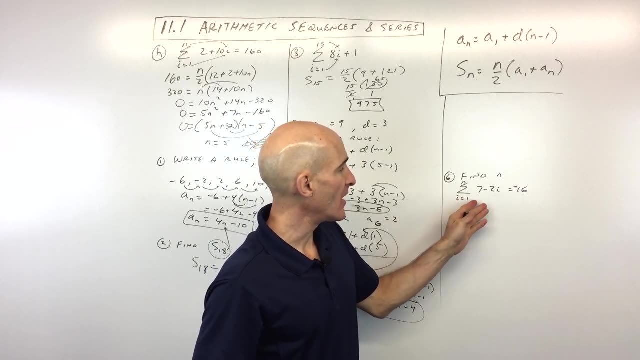 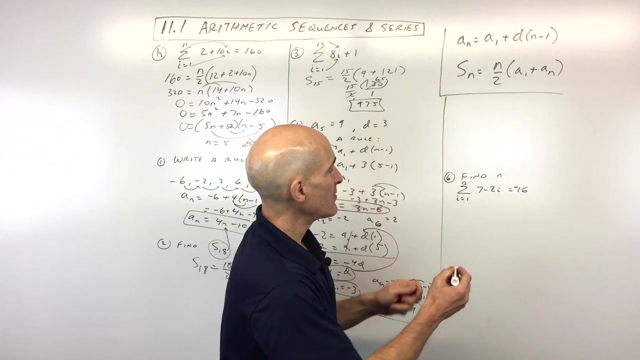 I first wrote it down. It's actually equal to negative 16. So what we're trying to do is we're trying to find this missing value n. This is the sum of the first n terms of this arithmetic series. And it equals negative 16. So how would you do that problem? Well, if I was going to do it, I'd be using this formula up here. I'd say that the sum is negative 16. There's n terms. We don't 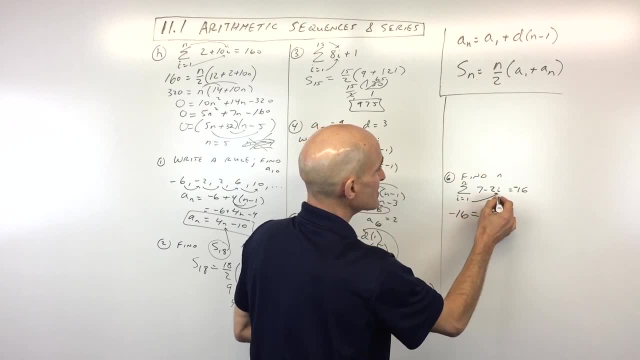 know how many. And the first term, if we put 1 in, we get 7 minus 2 times 1. 7 minus 2 is 5. 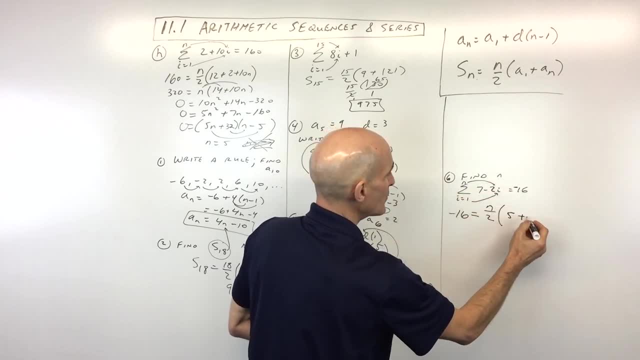 And the last term, the nth term, we don't know what that is. But if we put n in, we get 7 minus 2n. 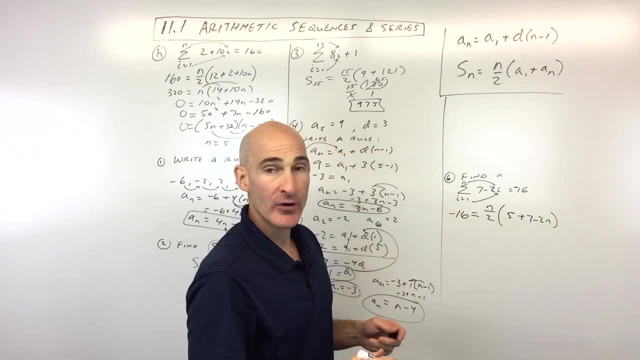 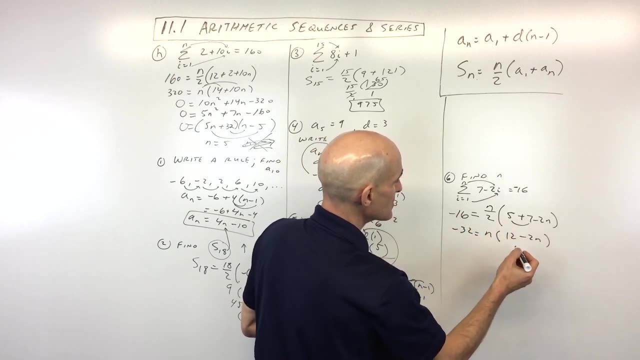 So we have an expression for the nth term. All I have to do is solve for n. I'm going to multiply both sides by 2. That comes out to negative 32 equals n. 12 minus 2n, just combining like terms. And then if we distribute the n, you can see we're getting negative 2n squared plus 12n. I'm going to add the 32 to the other side, set this equal to 0. I'm going to divide everything by negative 2, just to make it a little bit easier to factor or solve. And so now what we're going to do is we're going to factor and set the factors.